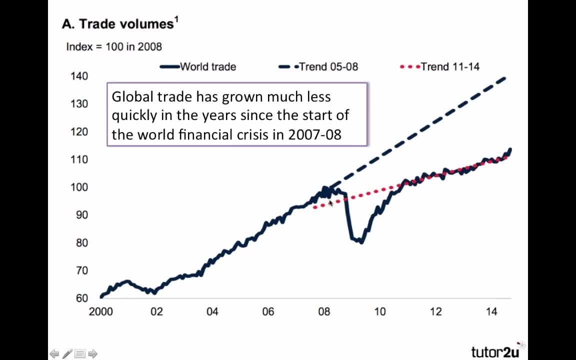 2007.. 2008 into 2009 and many countries going into recession. Look what happened to the value of world trade. It fell very sharply. It took us back almost 10 years to where we were before. Obviously, it recovered in 2010 and 2011. and what have you but notice the gradient of. 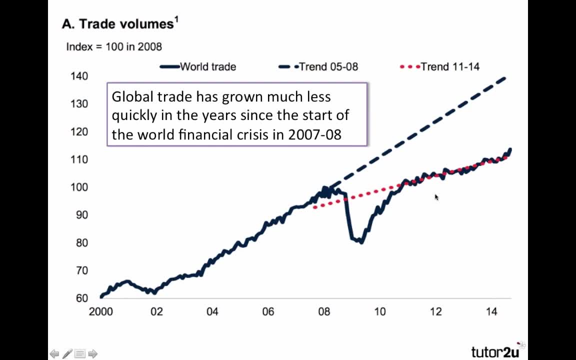 the red dotted line. That is the trend growth of world trade from 2011 to 2014.. It's much flatter than the previous trend, So I think we can say that globalisation is not inevitable, that trade normally increases most years, We seem. 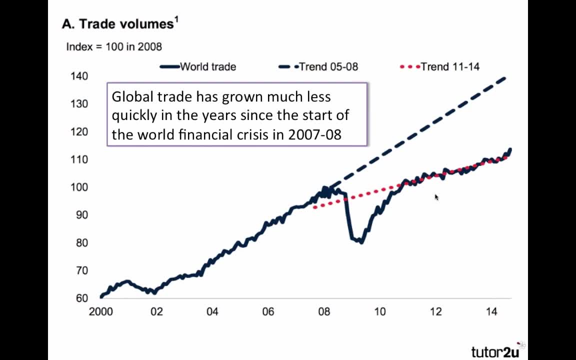 to be in a phase where world trade, the global exchange of goods and services- that's growing slightly less quickly than it was the previous decade. That gives you an idea of the impact of the shock of the world financial crisis of 2007-2008.. 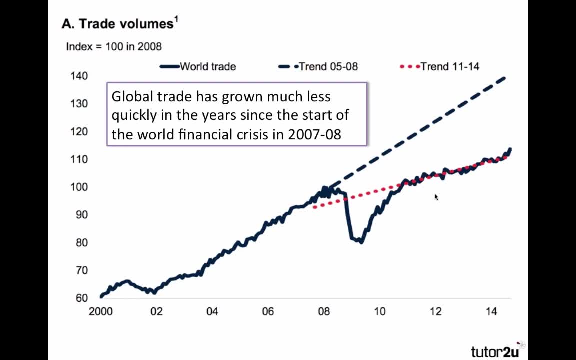 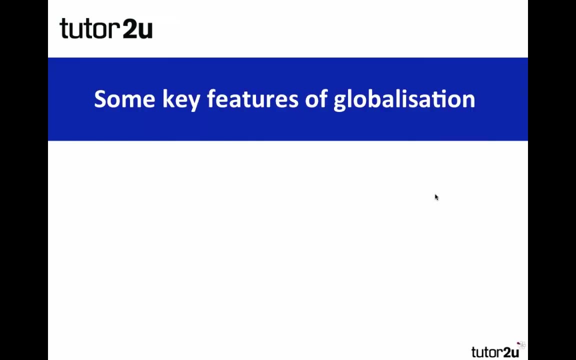 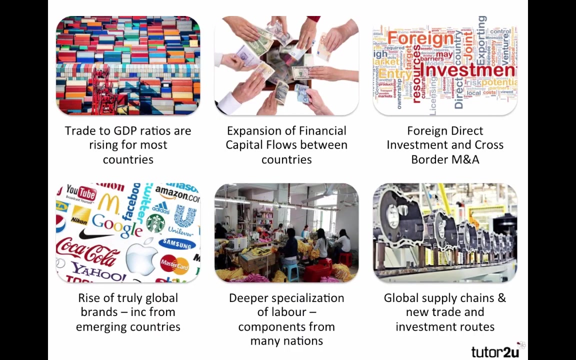 Also, I think what this chart also demonstrates is that, instead of globalisation of trade- true globalisation perhaps- we're moving into an era of regionalisation. Increasingly, you get intra-regional trade becoming a dominant force in the world economy. What are some of the key features or characteristics of globalisation? This slide tries, I think. 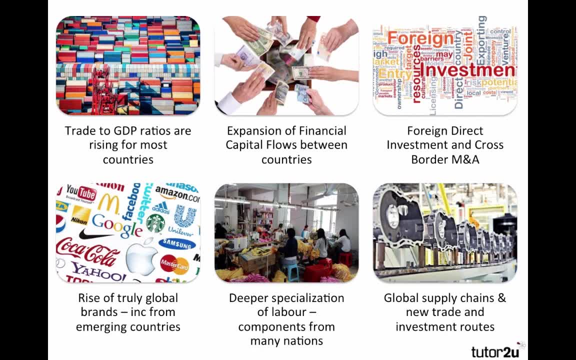 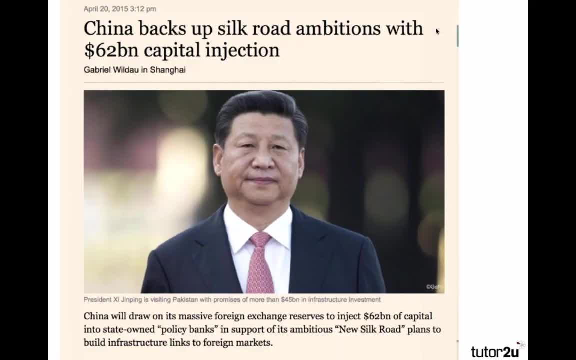 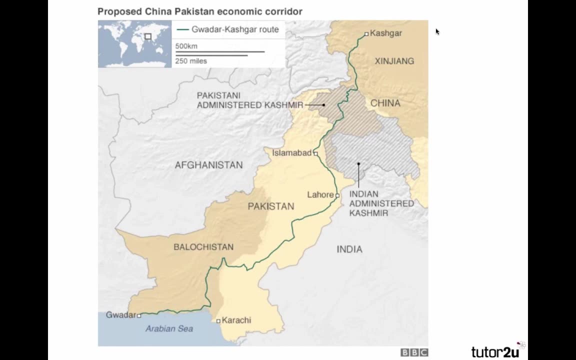 between China and the emerging world. Just a couple of days ago, China announced a $60 billion capital investment plan, including a huge plan to build a new economic corridor through Pakistan to the Arabian Sea. These are enormous, absolutely enormous plans. There's many, many barriers along the way. 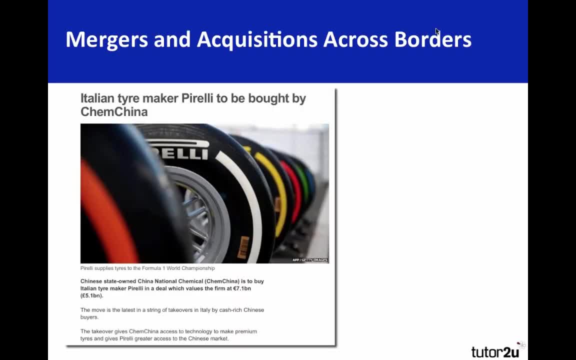 but this is a key feature of our globalizing world. And of course, I mentioned acquisitions. You don't have to turn very far in the newspapers to find examples of where Chinese companies are now buying up Western technology. So Geely buying the Swedish car firm Volvo. 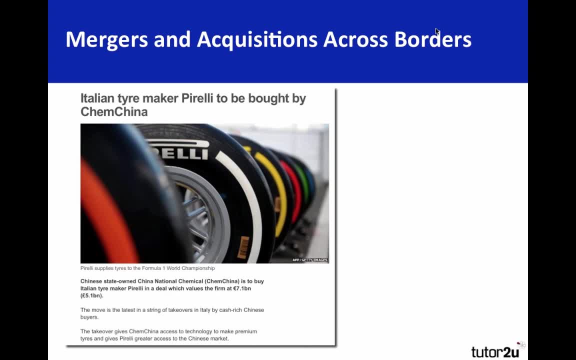 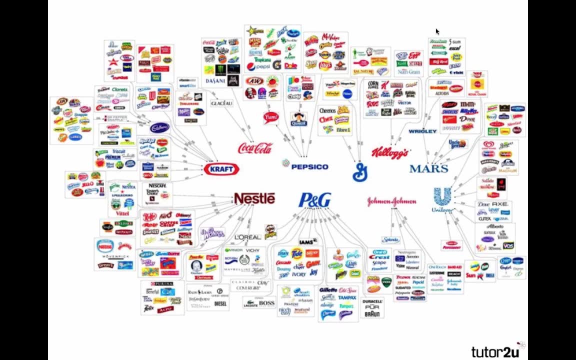 The Italian tire maker, the iconic tire maker, Pirelli, to be bought by Chem China. There are many, many more examples along the way. And, of course, globalization, for many of you, is the rise of the global brands. I love this graphic. 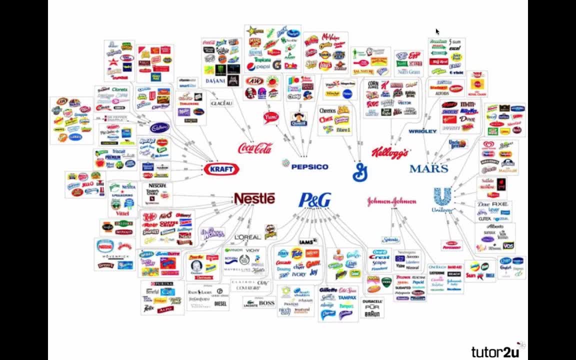 This graphic suggests that the 10 kind of leading consumer facing consumer goods and services companies have an incredible reach of the brands and the products that we consume. So, from Kraft to Nestle to Procter & Gamble, to Mars to Kellogg's. 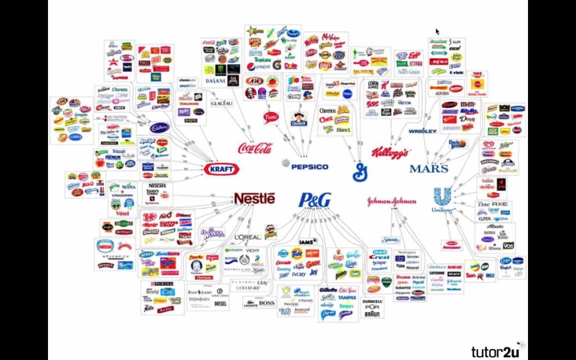 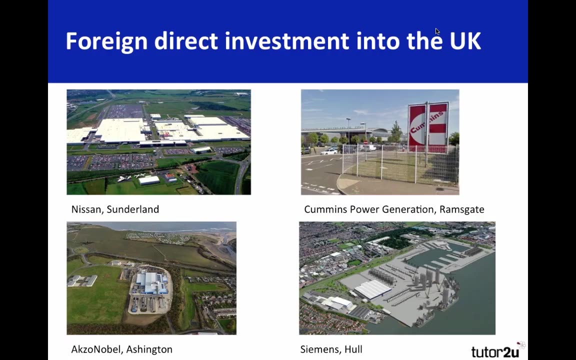 they literally satiate and swamp in many ways the retail malls with their products. This is the idea that globalization may or more precisely, have led to a loss of cultural diversity, a standardization of global brands. Foreign direct investment is important for the UK. 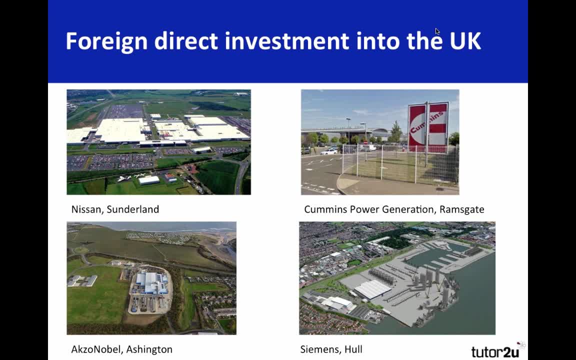 Everybody in the exam mentions Nissan. It's ok, it's top left on this chart, One of the world's biggest car plants. And just have one more example with foreign investment other than Nissan for your exam to demonstrate the advantages, for example, of FDI into the UK. 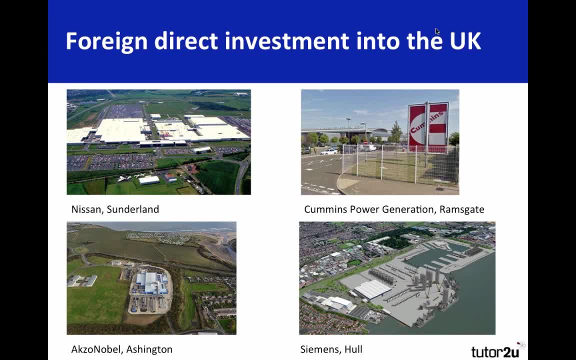 and very important in the hole at the bottom right there, The Cummins Power Generation Plant in Ramsgate. There are many, many examples. one could find The Axo Nobel Plant in Ashington in the northeast of England. Don't necessarily rely just on this app. 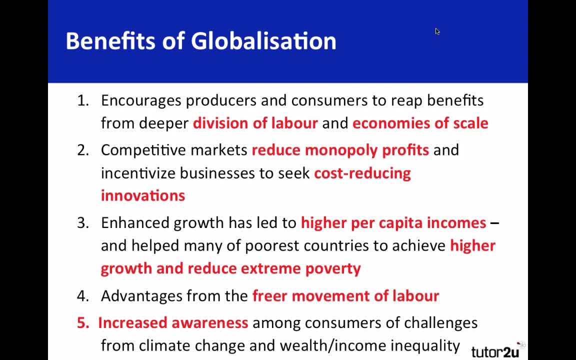 So let me take you through what I think are some of the key benefits of globalization generally. We'll come to the issue about the UK in a second or two. The key here, I think, is to be able to match some good, solid theory, some good analysis. 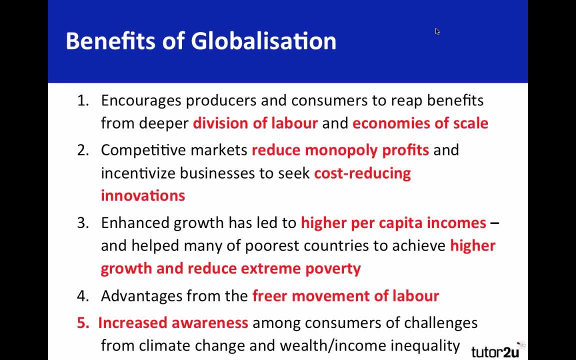 with what you see happening in the world and your experiences, And there's no right or wrong answer to these kind of questions. To my mind, fundamental benefit of globalization is that it allows consumers to benefit from what producers are doing. So the greater specialization, the greater division of labor. 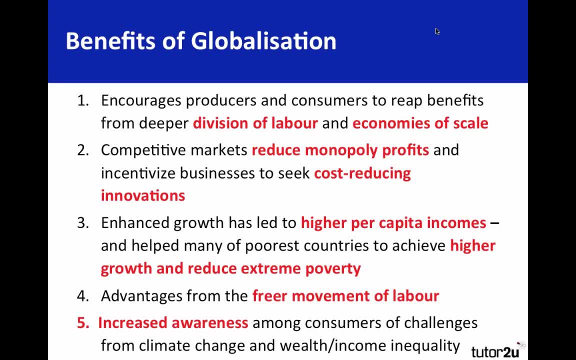 scale economies in theory should bring about consumer welfare gains. And if globalization is a benefit, big if, if it leads to more competitive markets, then again in theory that should bring down the rate of super normal profit of monopoly producers. 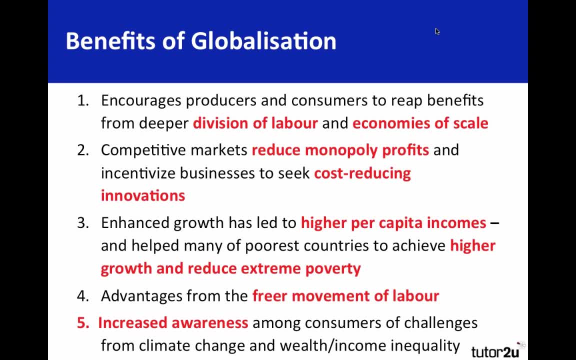 But also incentivize businesses to be more dynamically efficient and to kind of seek some cost-reducing process innovations in markets. Again, consumers stand to benefit there, because if profits are lower and prices are lower, then real incomes go up and the amount of consumer surplus. 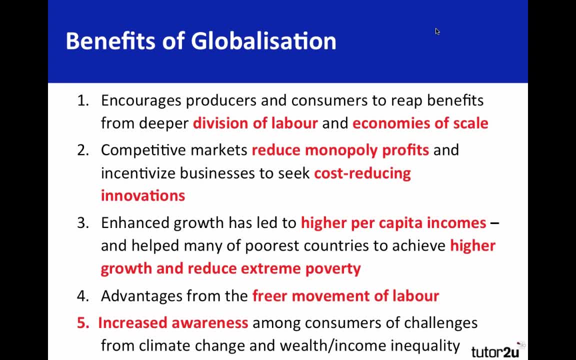 enjoy also rises. And if globalization leads to again to stronger growth of real GDP in the world- And keep in mind that the world economy grows up between 3% and 4% per year- And if that leads to faster growth. 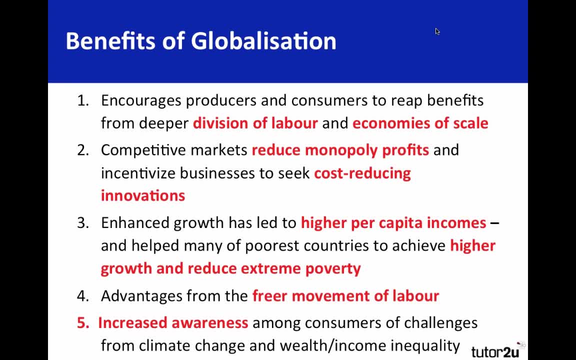 with a given level of population growth, that should help to lift per capita incomes and therefore bring down extreme poverty and achieve some of the Millennium Development Goals. My own view is that the free movement of labor is a positive. It's a benefit to many, many countries. 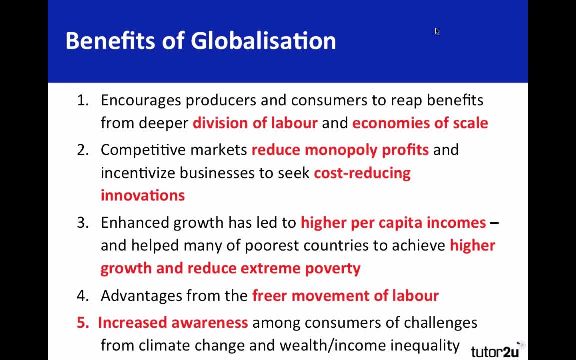 Thank you. And globalization, if it involves a greater degree of geographic mobility of labor, is another benefit. And one can argue in a slightly non-economic way that as people travel more and experience more of the world around them- students on gap years, people on sabbaticals, 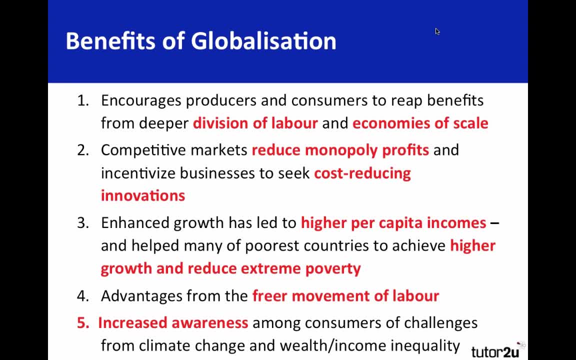 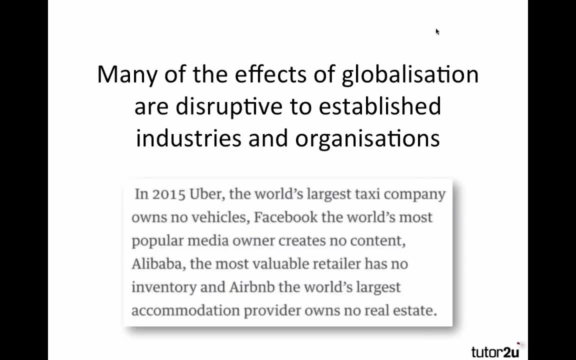 people traveling the world for business as well as for leisure, then they become much more aware of the global issues and the global challenges, ranging from inequality to climate change to democracy. I think that awareness is something which 15, 20 years ago really wasn't on the same level. 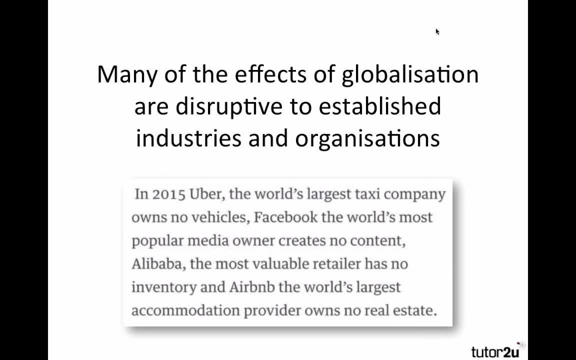 What's really interesting from a microeconomic point of view is that globalization is, in a sense, fast forwarding the disruptive aspects of new technology. I love this quote. It came from an analysis of creative destruction. I think it was from The Economist a few weeks back. 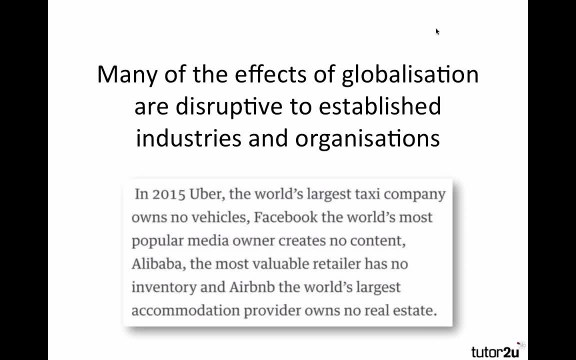 If you take four of these companies- Uber, it's become pretty much. It's become the world's biggest taxi company. It doesn't own a single vehicle. Facebook is a huge media company. It doesn't create any content. Alibaba has become the world's biggest retailer. 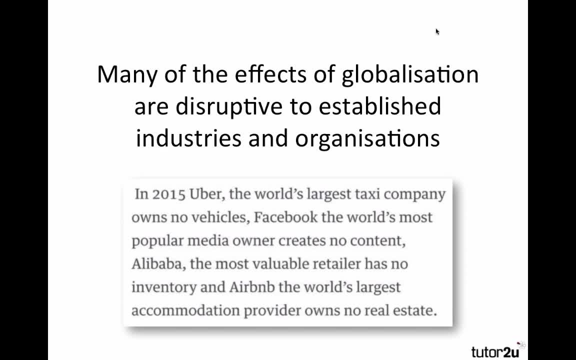 bigger than Walmart. It doesn't have any stock And Airbnb, in stock market terms, is probably worth more than Intercontinental Hotels or Hilton Hotels. It doesn't own any rooms, So globalization, in a sense, provides a platform and an opportunity for new companies to emerge. 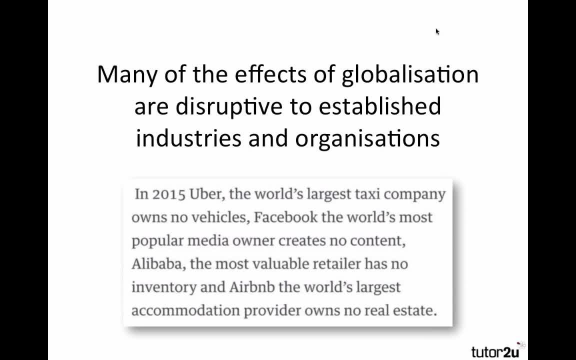 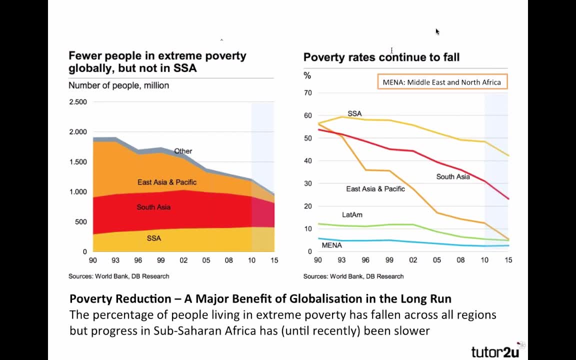 And for these companies. it's a great opportunity For these businesses to scale up at a speed which is unprecedented. Just a few bits of pieces in terms of the wider benefits of globalization. My own view is that globalization's helped significantly to bring down extreme poverty. 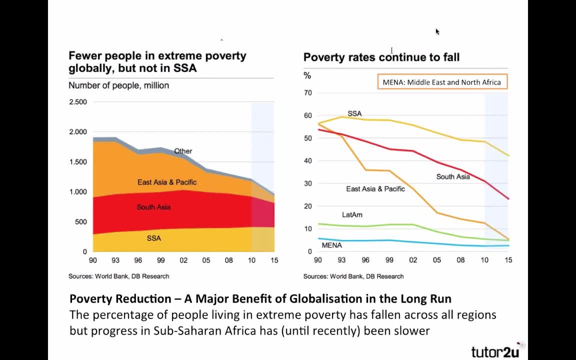 There are many, many fewer people living in extreme poverty. That's less than $1.25 per day PPP, But obviously progress in sub-Saharan Africa has been smaller than the number of people in sub-Saharan Africa who are in extreme poverty has gone up. 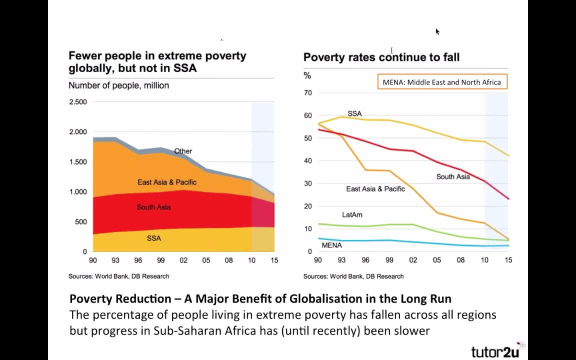 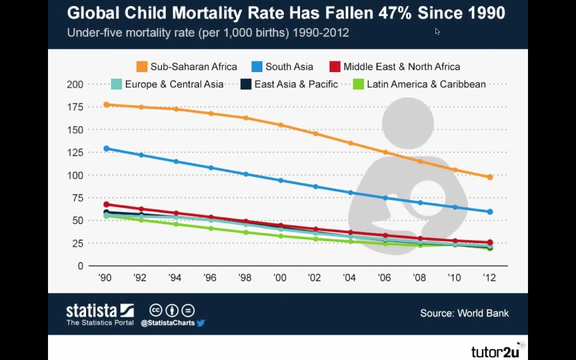 And that's largely on account of rapid population growth. But poverty rates are falling, albeit too slowly. in many cases, Child mortality has fallen. This chart's taken from the World Bank And, again, although sub-Saharan Africa is significantly well ahead, progress is being made in reducing. 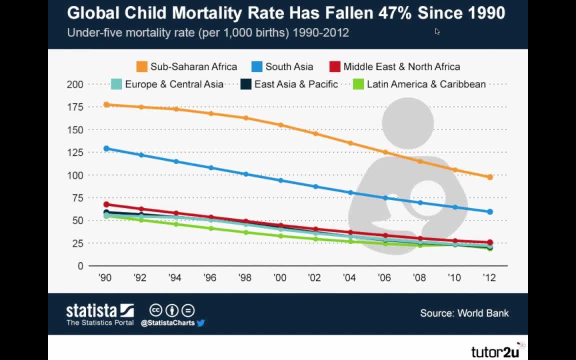 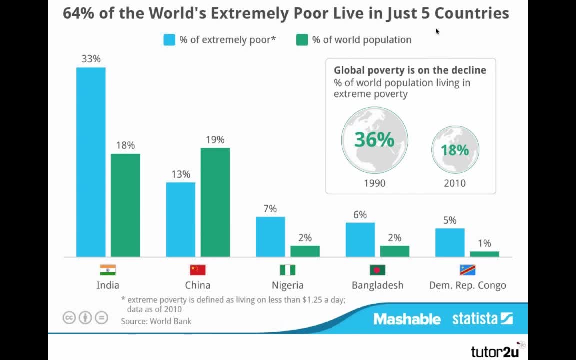 the rate of child mortality. Of course that's one of the key Millennium Development goals. That said, we still have countries, countries, countries, countries where the majority of the world's extreme poor live in only a few nations. So one can see here that the population 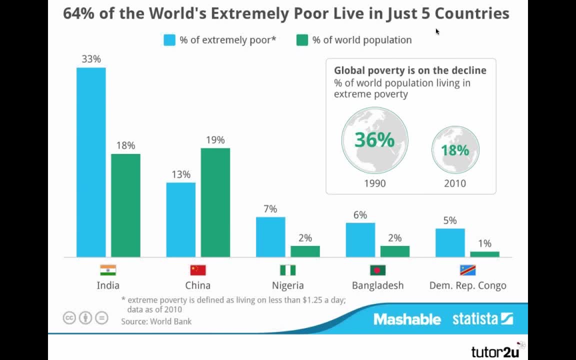 living in extreme poverty is half since 1990.. But two-thirds of the world's extremely poor live in just these five countries: India, China, Nigeria, Bangladesh and the DRC, And of course, all kind of issues we mentioned. 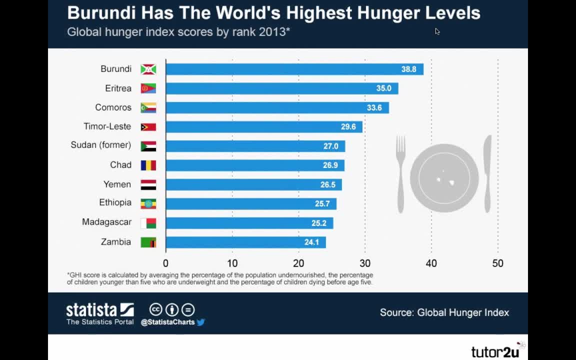 awareness of issues such as malnutrition, extreme hunger. each year we get the data published on the Global Hunger Index And I'm just giving you this slide, so you have a little bit of awareness of which countries, sadly, figure right at the top of this list. 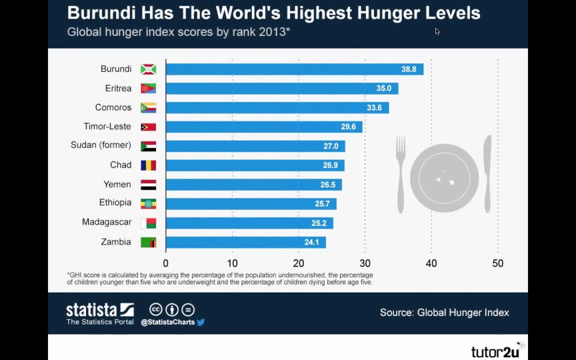 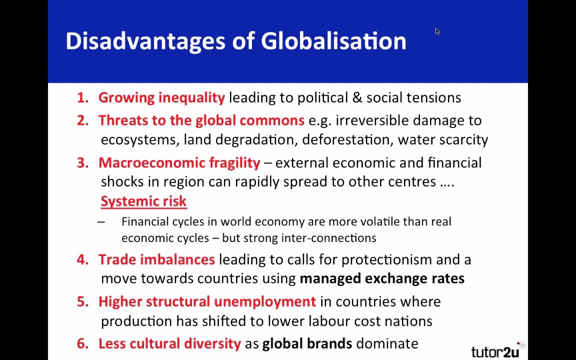 in terms of the percentage of the population who are measured as undernourished or underweight, Burundi and Eritrea are significantly above the world average and the average of some of the least performing countries. What about the disadvantages of globalization? Globalization- 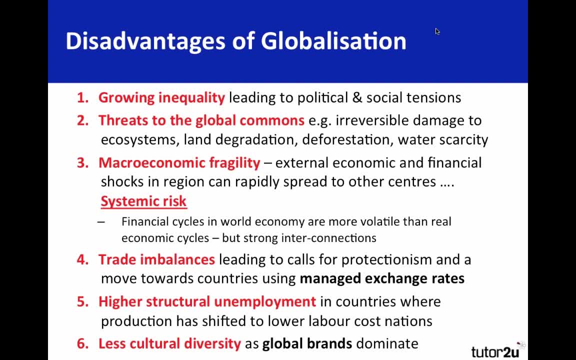 This is one of those topics that raises many, many different opinions And it's pretty hard to avoid making value judgments. I'll do my best, but can I try and pick out a few broad examples of disadvantages? One is the issue of whether globalization 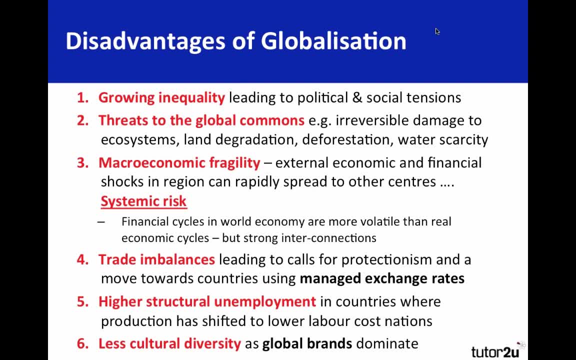 whilst lifting per capita incomes and reducing extreme poverty might also be a factor, a catalyst, behind increasing inequality of income and wealth Within countries. I think it's one of the paradoxes of globalization that globalization has reduced inequality between countries, but may well have increased it within nations. 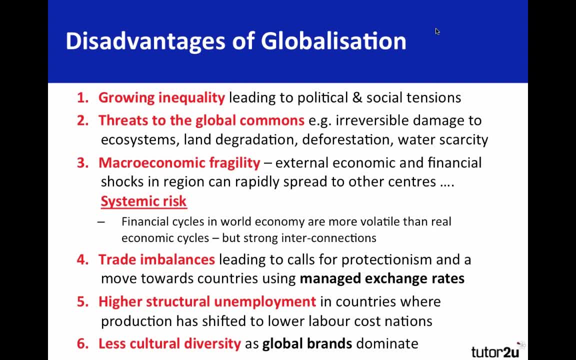 Second disadvantage relates firmly on the environmental aspect. We see, as world output and world trade increases, we see some of the consequences for carbon emissions, for loss of biodiversity, for increasing water scarcity and the loss of natural capital, which clearly is a threat to the global commons. 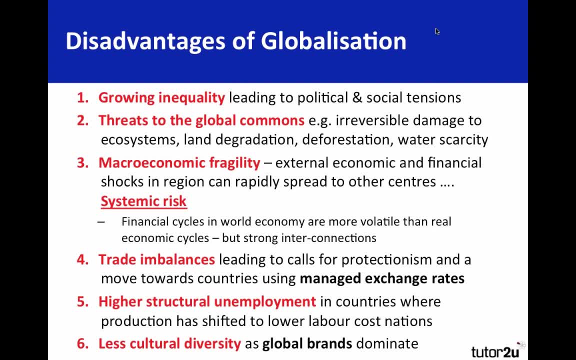 The third point I want to make is that globalization, which I've defined as a more interconnected, interdependent world, whilst that can help make countries more resilient because, for example, they might be trading with many more countries, actually it's a process which could make countries more fragile. 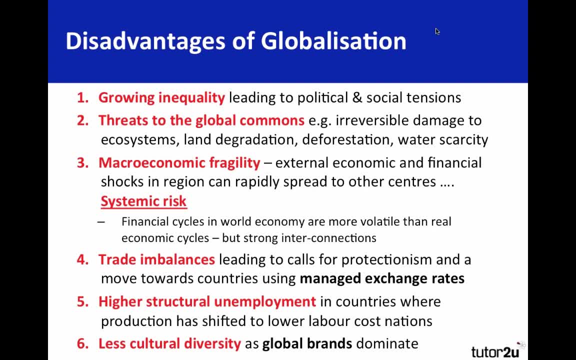 The key words here, which I've underlined in red, are, for example, systemic risk. Events in one part of the world could have a reverberation effect thousands of miles away. So an external shock, a fall in the price of oil. 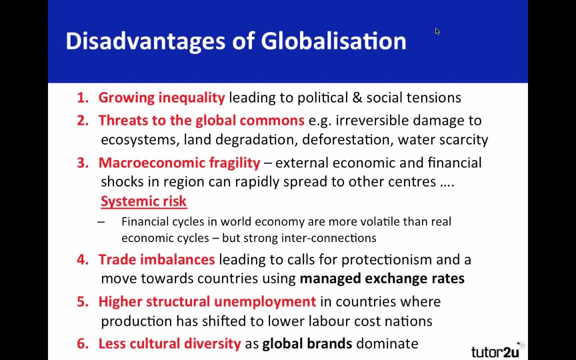 a collapse in the price of iron ore or stock market volatility in one country, they can have significant externality effects which bring about systemic risk. The evidence is pretty strong that financial cycles changes in asset prices, exchange rates and credit those cycles. 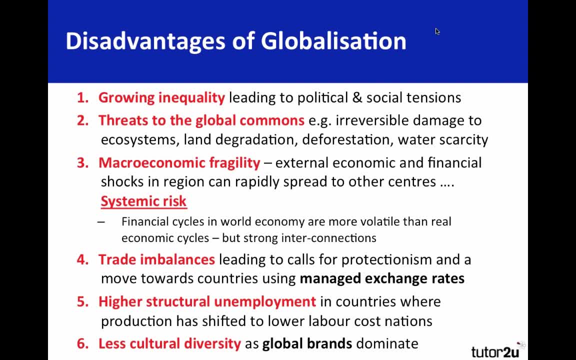 are more volatile than real cycles- cycles of output and jobs investment. There's very, very strong interconnections between them. I'll come back to that in a second. Trade imbalances are also an important disadvantage of globalization. Increasingly, we see in the world the rise. 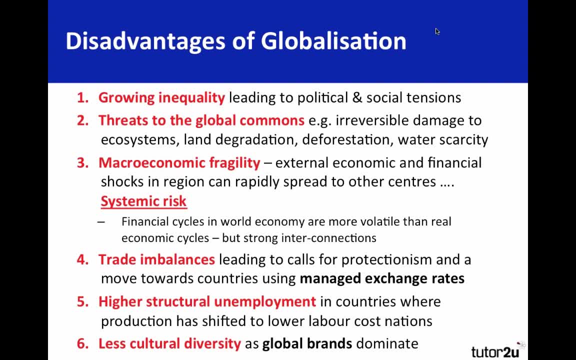 of mega surplus countries, countries running current account surpluses in excess of 10% of GDP. Two examples: there would be countries such as Singapore and Norway, huge surplus countries. Until recently, Saudi Arabia would be there until the price of oil collapsed. 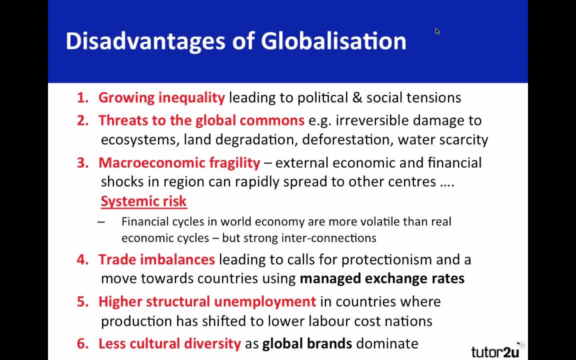 And yet we also have countries running enormous trade current account deficits, of more than 8% to 10% of GDP, including many countries in sub-Saharan Africa, Kenya, Ethiopia, Ghana. So trade imbalances are becoming a feature of globalization And with those, come calls and political pressure. 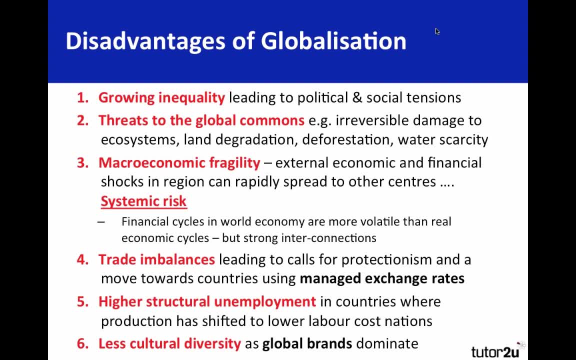 the tariffs and quotas and other forms of protectionism, and also, increasingly, countries avoiding using free-floating exchange rates and deciding to move to more managed exchange rate systems. Many countries, although incomes have gone up, although GDP has gone up, structural problems. 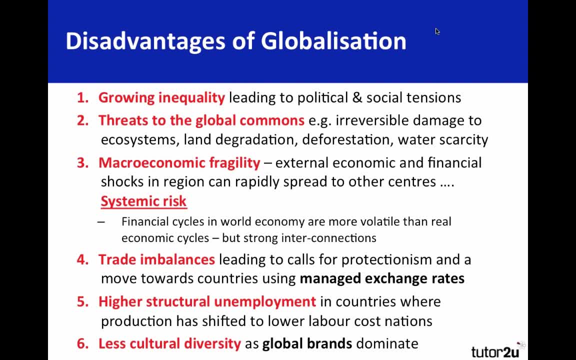 have emerged, Manufacturing has shifted to lower labor cost nations, Other industries have declined and that leads to structural unemployment, a major cause of labor market failure and a big policy issue. And there's the issue about global diversity- cultural diversity. Are global brands dominating the landscape in too many countries? 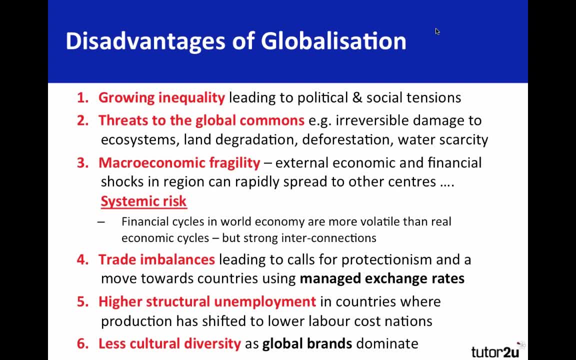 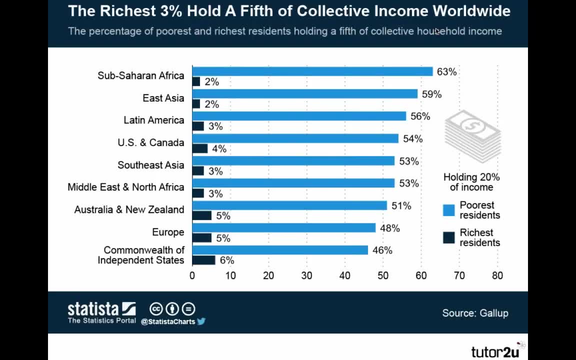 Are we losing out on the smaller businesses, the bespoke businesses and the products they produce? Here's a few more charts on globalization, most of which, I think relate really to inequality And, according to the Gallup, the richest 3% in the world. 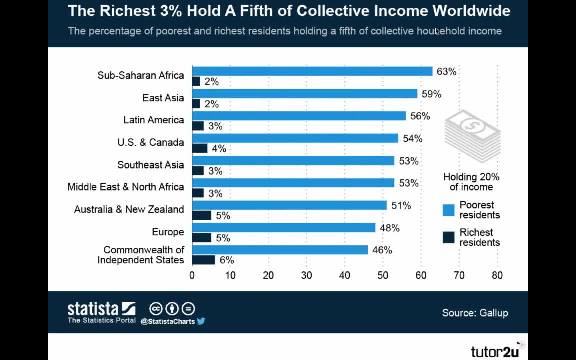 hold a fifth of all the income in the world. That's a lot. And if you look at sub-Saharan Africa, the richest 2% of residents hold 20% of the income, whereas 63% of the population only have 20% of the income. 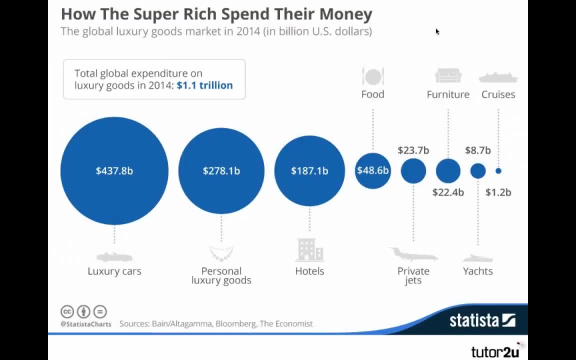 There's a huge gap between rich and poor, The rise of the super rich. This is taken from a survey by the management consulting company Bain And it looks at the spending of the super rich and how they spend their money on luxury cars, luxury. 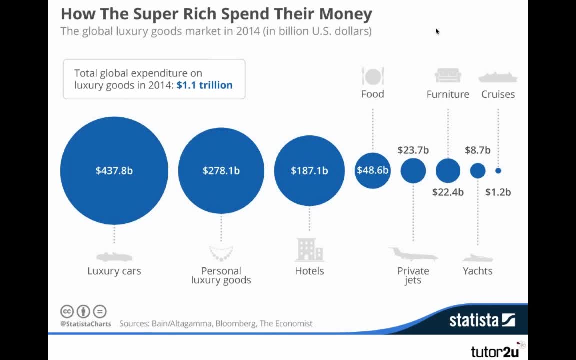 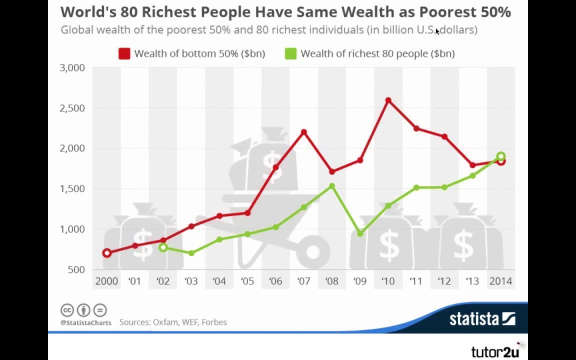 consumer goods: luxury hotels, jets and yachts- Incredible numbers Survey came out last year, a very well-known survey from Oxfam which said that the richest 80 people in the world- they could actually fit into a London double-decker bus. 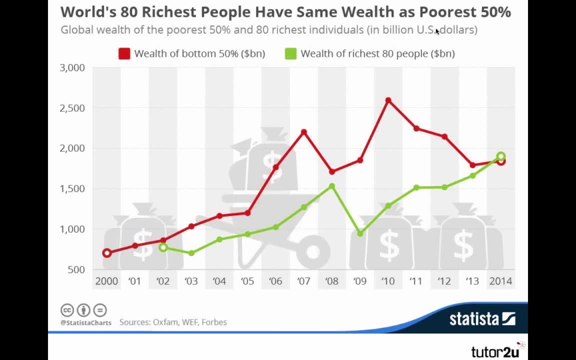 They actually own more wealth than the poorest 50% of people on the planet. Again evidence of the gap, the chasm in wealth between rich and poor. And here's the chart. I was trying to find it a few seconds ago. 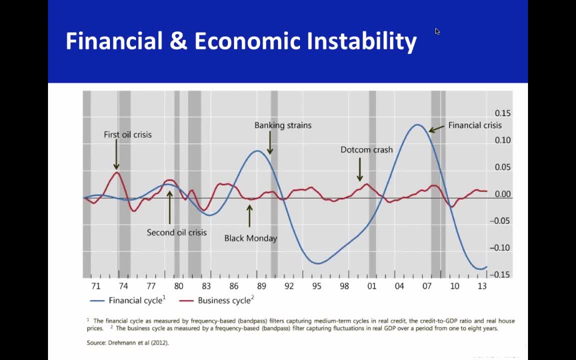 which shows the economic cycle in red- so-called business cycle, real GDP and financial cycles. Notice that those financial cycles seem to be getting more volatile, And they're certainly more volatile than real cycles. This is a major threat to the world economy. 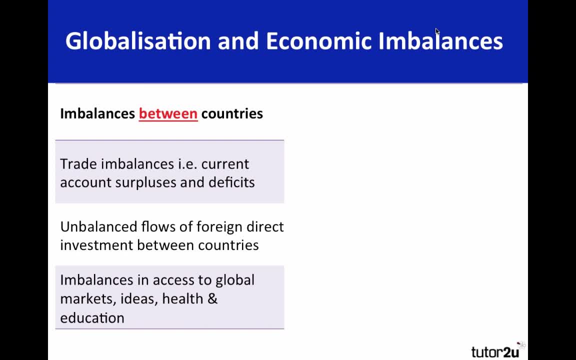 One of the key words I would be using if I was revising globalization and writing about it would be this word: imbalance. What we're seeing happen with globalization is growing imbalances, And there's two types. One is an imbalance between countries, a trade deficit. 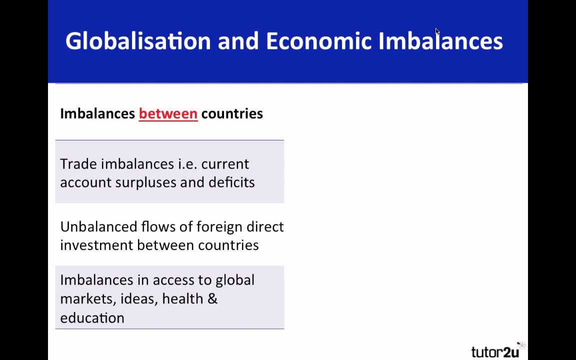 for example. So Norway running a 10% current account surplus, whereas the UK is running a 5% deficit. We see big imbalances in foreign investment between countries. Some countries are awash with FDI, Others struggle to attract anything like a significant capital inflow. 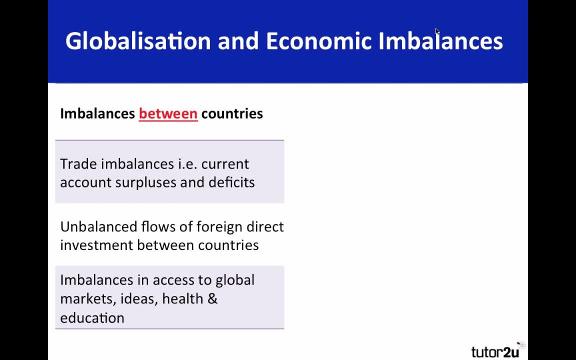 And we see huge imbalances within between countries in access to basic merit goods and basic public goods, Such as a decent education and an affordable health care system. And then we also have imbalances within countries. So the debate about inequality within the United States. 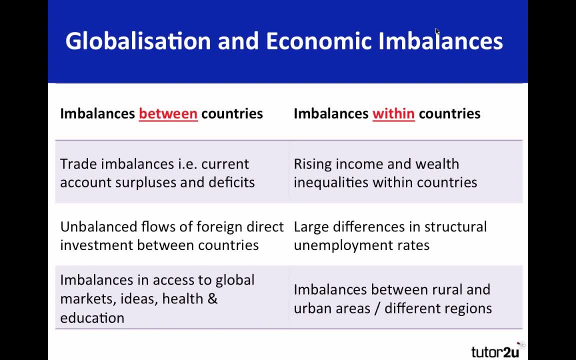 and the Occupy Movement is an example of that. If you take the UK, there are huge differences in unemployment rates across the regions. Higher unemployment in the Northwest, the Northeast and also in London. much lower unemployment rates, employment in some of the southern counties of the UK In countries such as China, the. 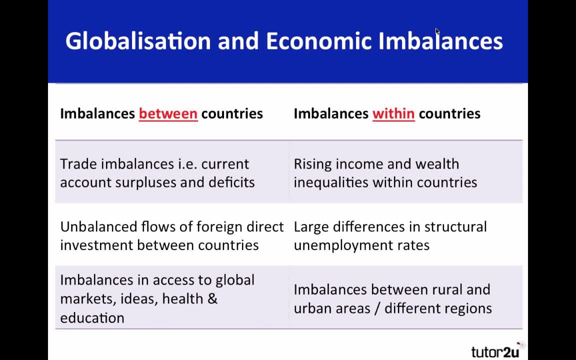 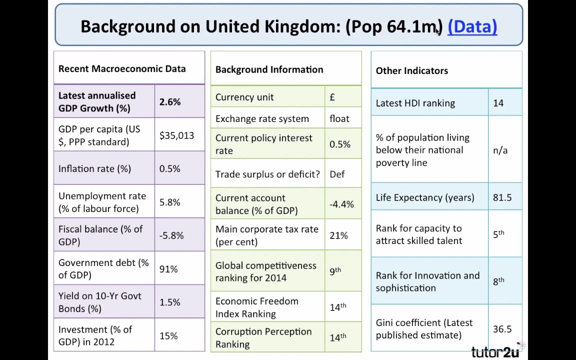 gap between rural and urban areas is also a major political issue. Globalisation could well be leading to bigger imbalances, and those imbalances are a threat to the globalisation process. The UK as a whole is pretty competitive. I'll leave this slide up for a few seconds. 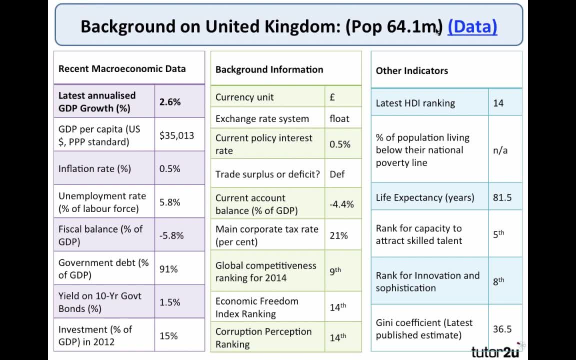 it's one of my country profile slides that I produce and we'll put some of these more on the website UK globally. if you look at the middle column, here go two thirds of the way down. Britain is ranked ninth globally in terms of competitiveness, Also ranked pretty. 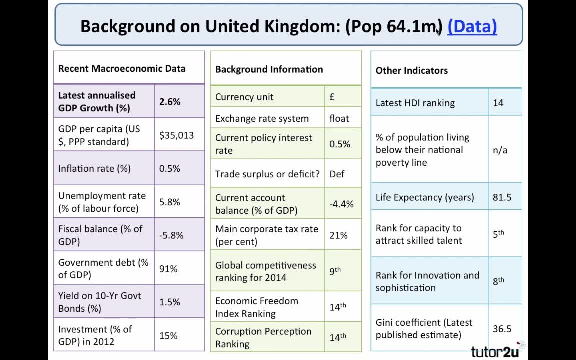 highly in terms of corruption perception. we have a pretty transparent economy, So Britain is fairly competitive in the world economy and that's a really good indicator to use. It leads us into a discussion about whether globalisation has been good or bad, or whether 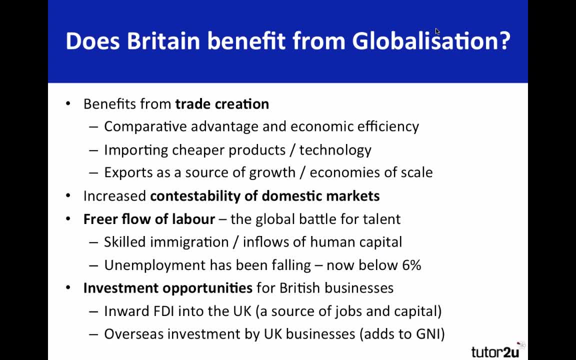 it's been bad for the UK over the years. So does Britain benefit from globalisation? Well, I suppose the quirky answer is: it doesn't matter. they can't avoid it. We're an open economy, we're open to trade, we're open to investment, and unless certain parties get, 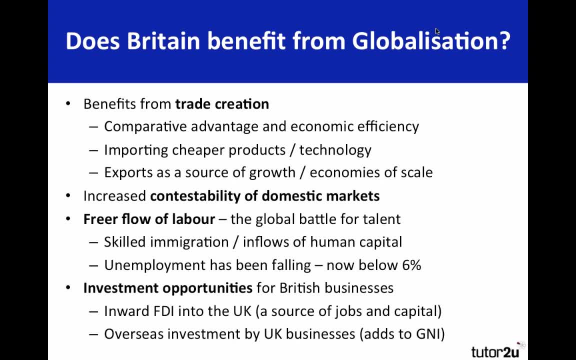 elected. we're open to the free flow of labour and capital. So Britain by and large, in the long term, benefits from the trade creation effects of membership of the European Union and wider participation in international markets. It allows consumers ultimately to benefit. 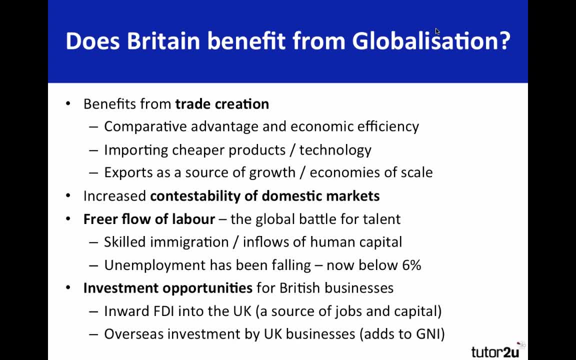 from the exploitation of comparative advantage. In other words, you can import cheaper products and new technologies, And exporters benefit from access to overseas markets as an injection of demand into the circular flow, allowing them to achieve economies of scale. Globalisation makes our markets more competitive. To use a micro term, it makes them more contestable. 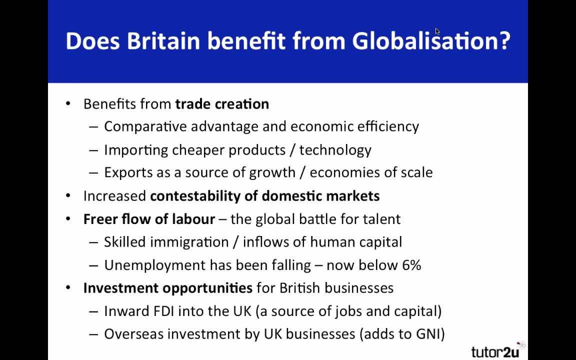 In theory that brings prices down and should drive unit costs lower. I think I argue that Britain benefits fundamentally from a freer flow of labour. There is a global battle for talent for the really highly skilled, highly motivated people, And Britain does. 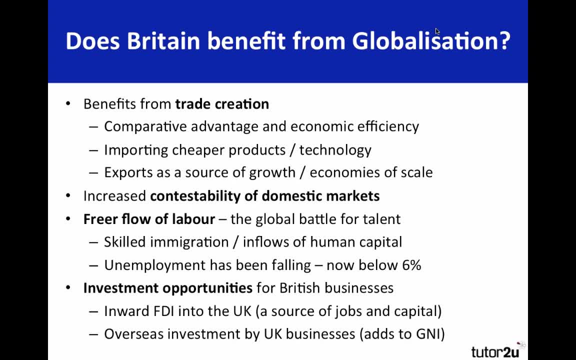 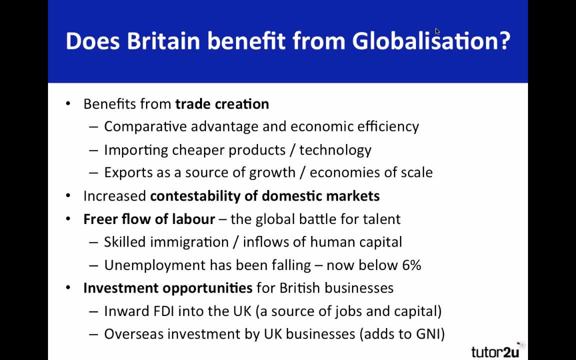 And for businesses in the UK it's a big problem. Evangelisation provides huge opportunities for investment. Lots of British businesses export overseas and invest overseas, And Britain is also a major attractive venue for FDI, which is ultimately a source of jobs. 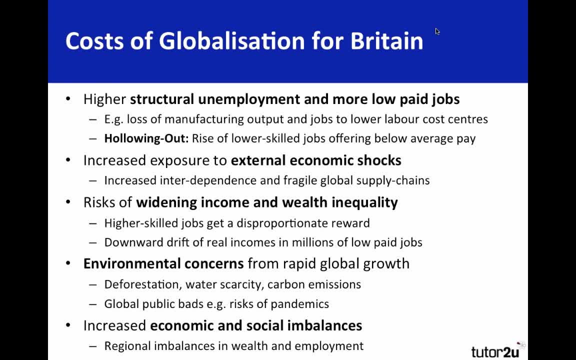 and capital, especially helping our balance of energy. On the other side, though, there are some risks, there are some costs from globalisation, But it's important to ignore them, as many people have a sort of tension when they think about what globalisation is doing to their lives. 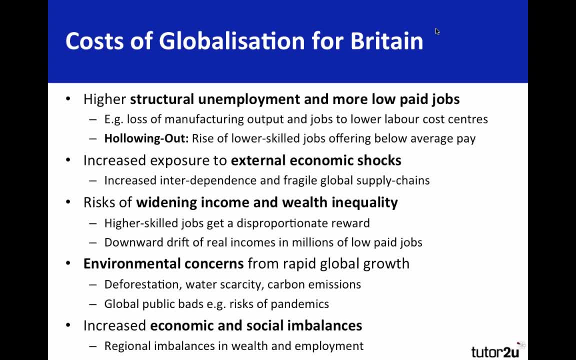 There is a danger that globalisation can lead to higher structural unemployment and more low paid jobs. I talked a few minutes ago about the hollowing out process. We've lost a lot of manufacturing jobs, particularly to lower labour cost countries in Eastern Europe and in the Asian continent, And so we get a hollowing out effect. We're left. 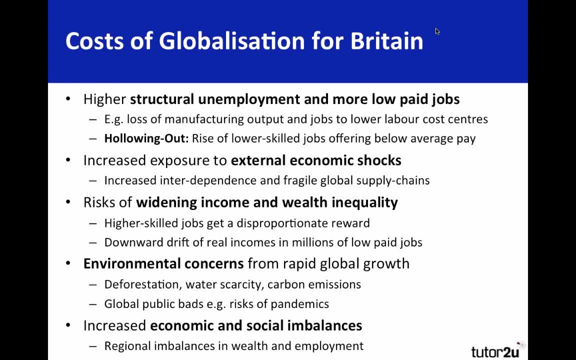 with many low skilled jobs, particularly in the service sector, that offer well below average pay, often times close to the minimum wage, And yet we also have a rising number of very highly paid jobs to which not everybody is able to get those kind of jobs. 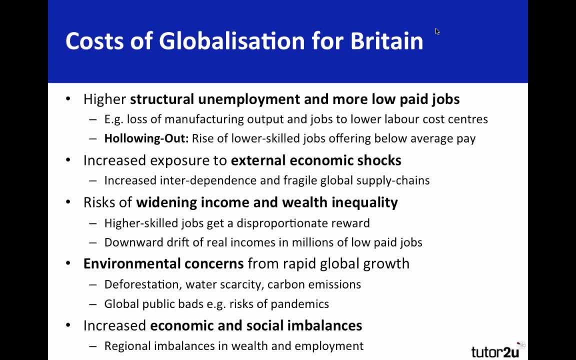 Britain benefits from globalisation because the world economy is growing but we are becoming more exposed to those external economic shocks, And interdependence of fragile supply chains can make the world a pretty tough place to do business, particularly when you get a global financial crisis. Globalisation could be leading to inequality, particularly the downward.